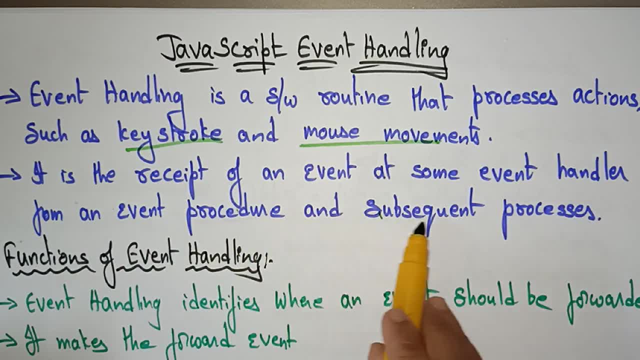 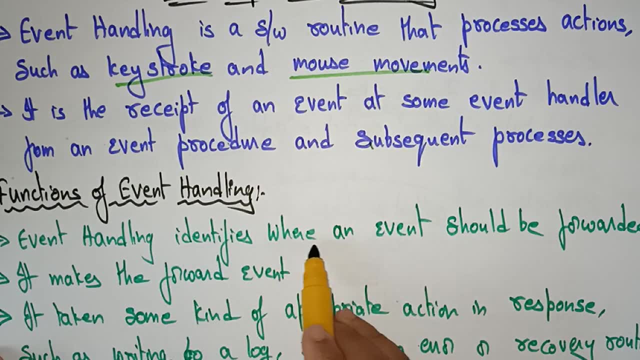 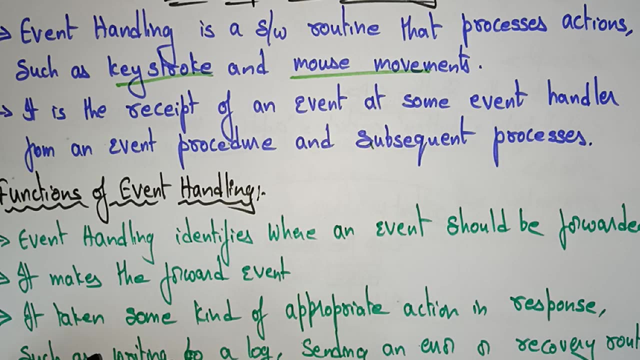 Let's see some of the functions of the event handling. The event handling identifies where an event should be forwarded. So you are doing some function, you are doing some activity, like you are doing some keystrokes or you are doing some mouse movements. So this event handling is going. 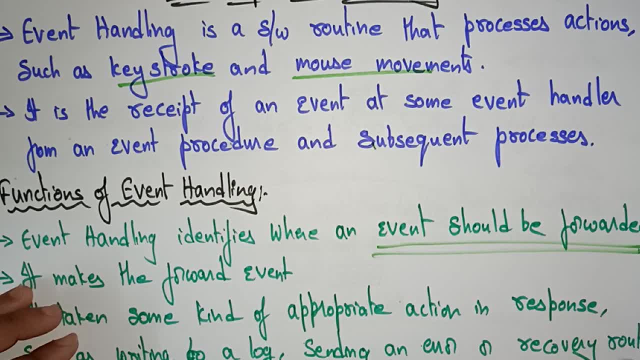 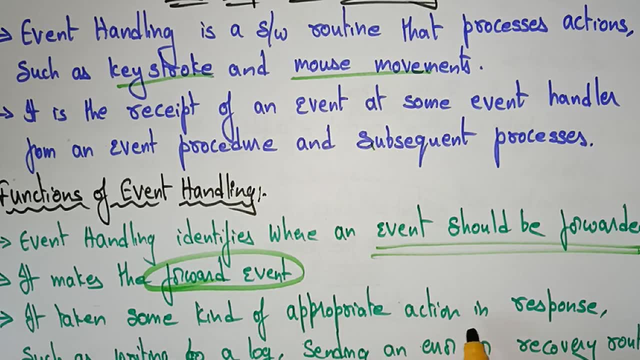 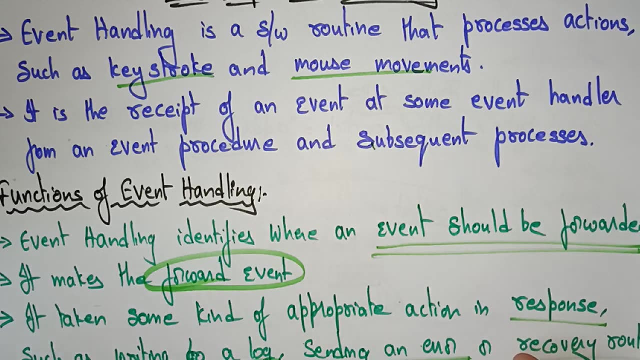 to be identified where an event should be forwarded. where I need to be forwarded, It makes a forward event. also, It takes some kind of appropriate actions in response, such as writing a writing to a logo, sending an error or recovery routine. So, like that, these are some appropriate actions that is doing. 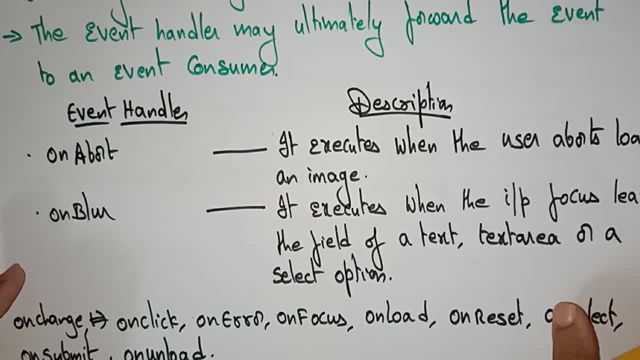 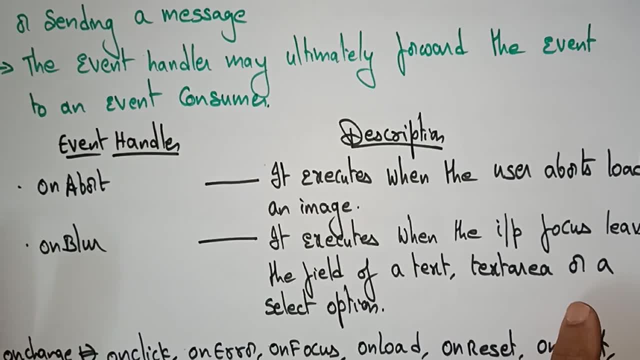 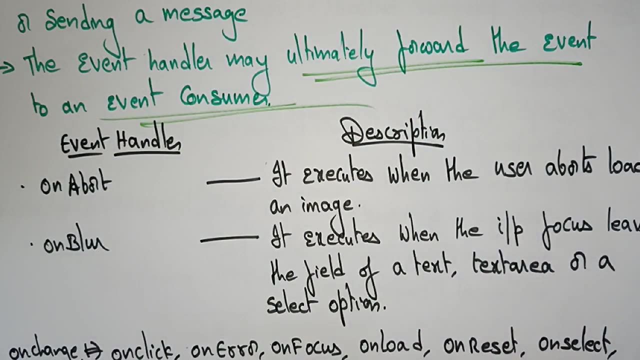 by this event handler or simply sending a message. also, The event handler may ultimately forward the event to an event consumer. That's the main goal of this event handler: It ultimately forward the event to an event consumer. So let's see some of the event handlers. So one of the event. 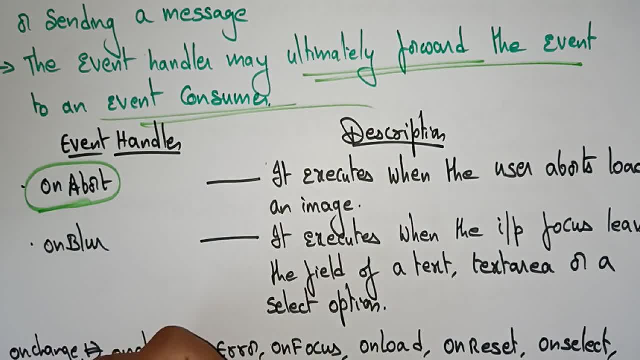 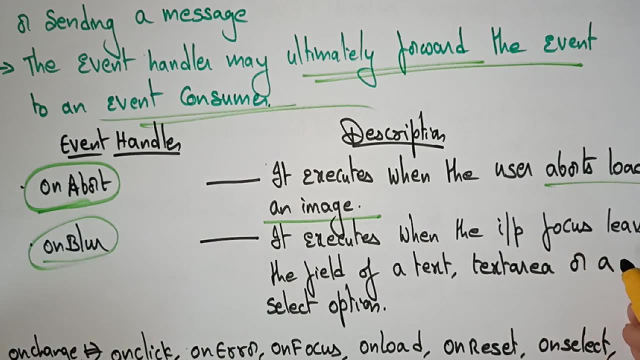 handler is on abort, on about means. it is doing some work. what is it is doing? it executes when the user abort loadings an image. users aborts loading an image on blur. it executes when the input focus leaves the field of a text or a text area or a select options. so these are different. 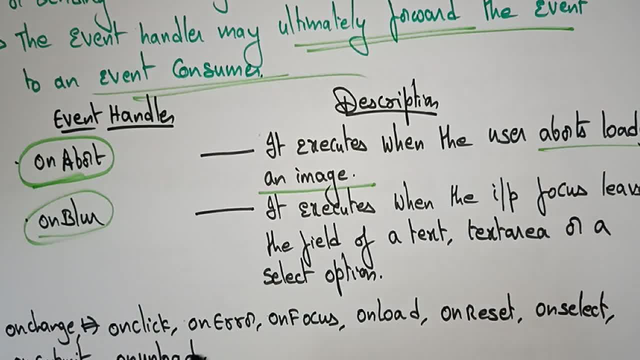 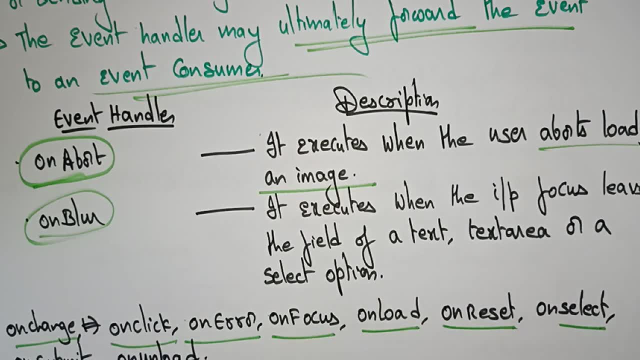 event handlers that we used and some more event handlers like on change, on click, on error, on focus, on load, on reset, on select, on submit, on unloaded. so many event handlers are there. so here, everything every event handler is going to uh is just a software routine that process the actions. 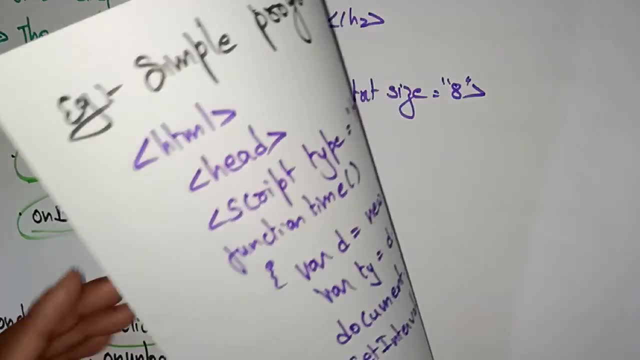 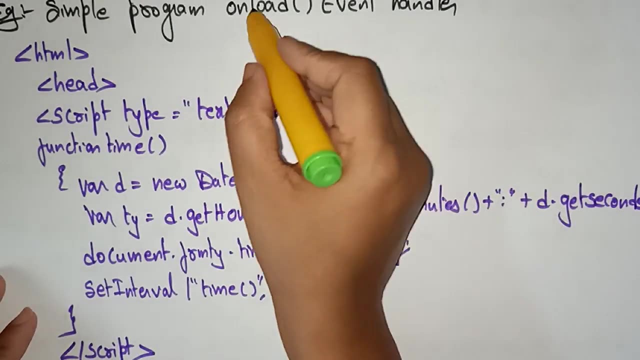 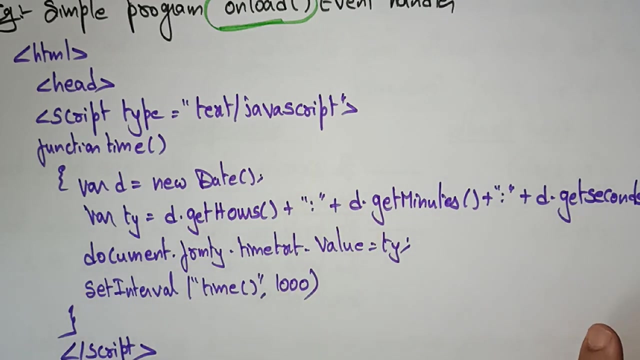 okay, every event handler is processing some action. let's see a simple example for this event handler, the simple program. i am taking one of the event handler like onload. let me take this as an example: onload event handler. so what this is going to. let's see, by using this event handler, what will be the output. 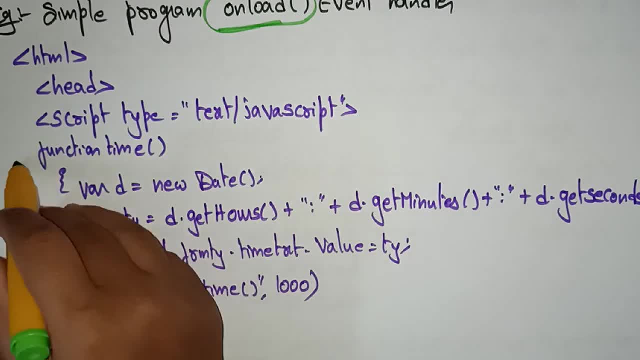 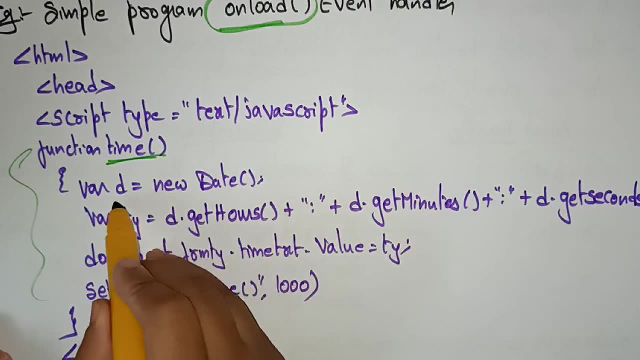 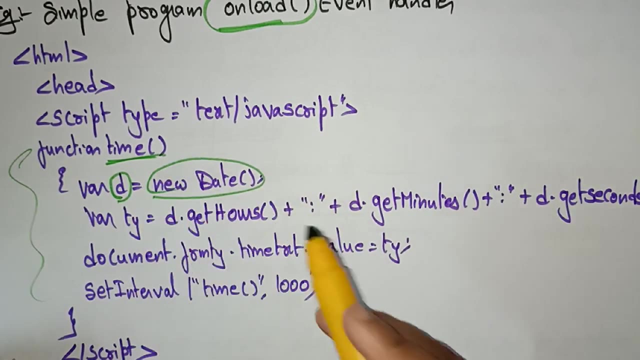 html head. in the head section i'm just writing the function, that is, a function time, a time i'm giving as a function name. so variable d is equal to new date. i'm assigning uh for one variable. i'm taking d. so for that variable d a new date is assigning. so at present,